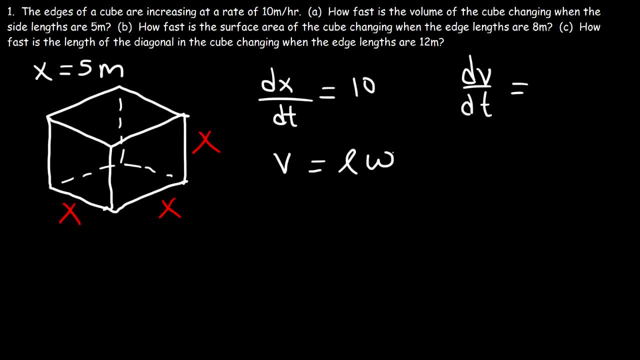 of a rectangular prism is the length times the width times the height. In this case, the length of the cube is x, the width is x and the height is x. So x times x times x, or 1 plus 1 plus 1, is 3, so the volume is x cubed. So now that 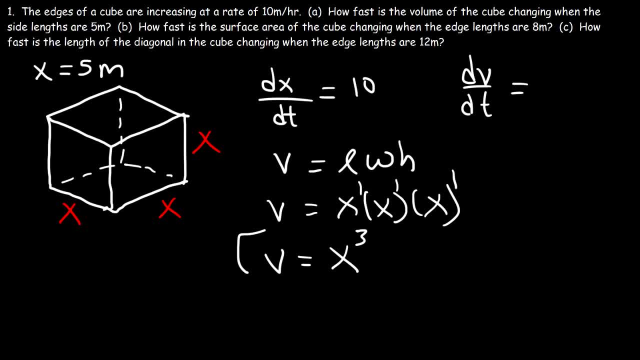 we've related v to x. we can differentiate both sides of the equation with respect to time. So the derivative of v is going to be 1 times dv- dt And the derivative of x cubed using the power rule is 3x squared times dx- dt. 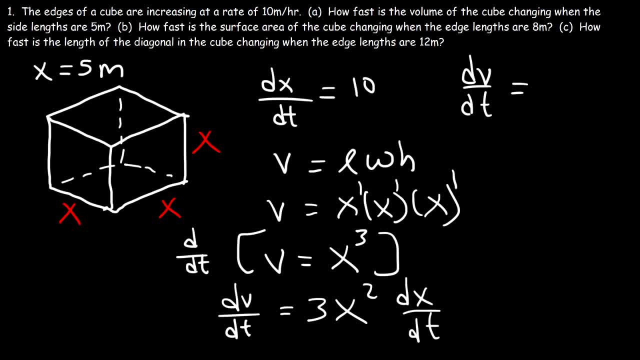 So that's the formula that we need to use right now, But let's get rid of some stuff. So we can see that x is 5 and dx dt is 10 meters per hour. So this is our equation, And we need to multiply it by the dot vector of dx. 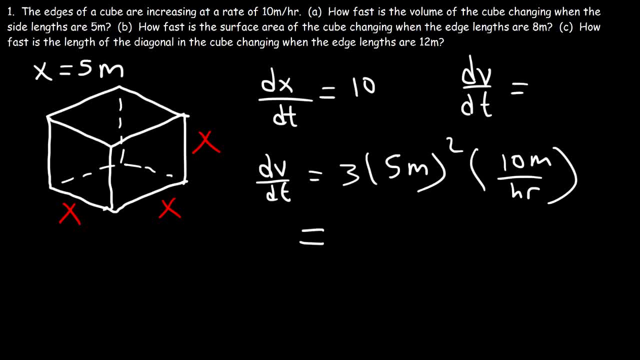 And we need to multiply it by the dot vector of dx. So this is our equation. So let's do that again. So that's the formula that we need to use right now. Now let's do the math: 5 squared is 25, and 3 times 25 is 75, and 75 times 10 is 750.. 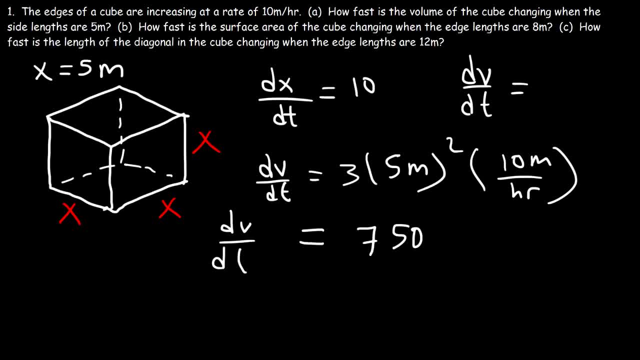 So dvdt is equal to 750.. Now, what are the units for dvdt? So notice that we have meters squared times meters per hour. Meters squared times meters, that's going to be cubic meters, So it's cubic meters per hour. 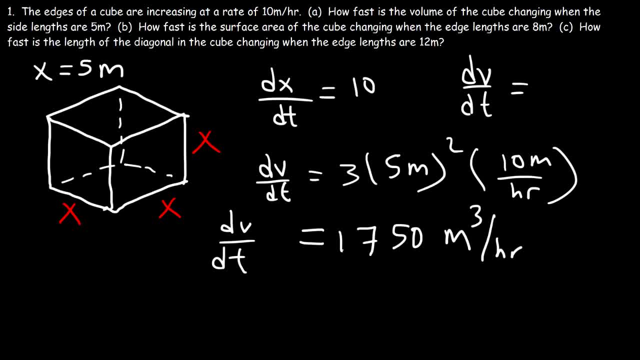 And since the edges of the cube are increasing, dvdt is increasing, so it's equal to a positive number. And that's it for part A of this problem. So that's how you can calculate the rate at which the volume of a cube is changing. 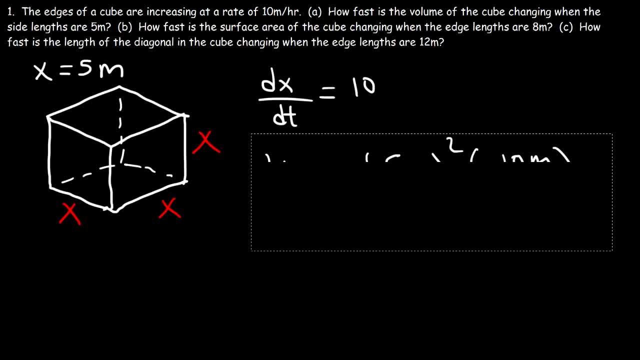 Now let's move on to part B. How fast is the surface area of the cube changing when the edge lengths are 8?? So x is no longer 5, but it's 8 meters. So let's change that number. So how can we find the answer to this question? 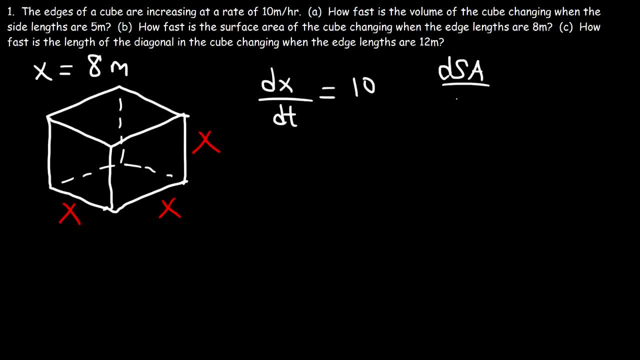 How can we determine the rate at which the surface area is changing? How can we find dsadt? So first we need to come up with an equation that relates the surface area. The surface area is going to be the area of all six sides. 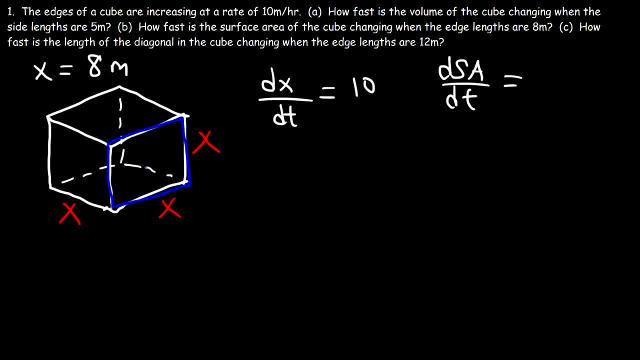 So notice that we have a side in the front and one in the back, So that's two sides. Here's the one on the left and here's the one on the right, So that's four sides. And then we have the bottom face of the cube and the top face of the cube. 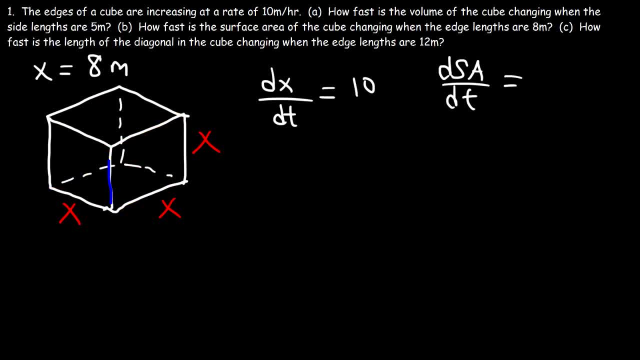 So there's six faces. Now the area of each face, the area of a square, is the left times, the width, or simply x squared, So the surface area of the cube, because there's six faces, all of which are going to be the. 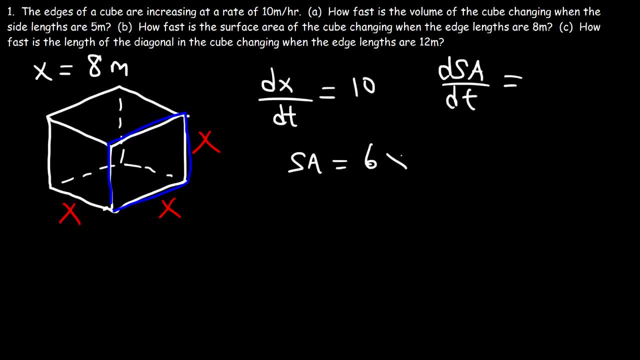 same. it's going to be 6 times x squared, Because you have to add up the area of each face, Each of which is x squared. Now let's find the derivative of both sides of the equation with respect to t. So the derivative of sa is going to be 1 times dsadt. 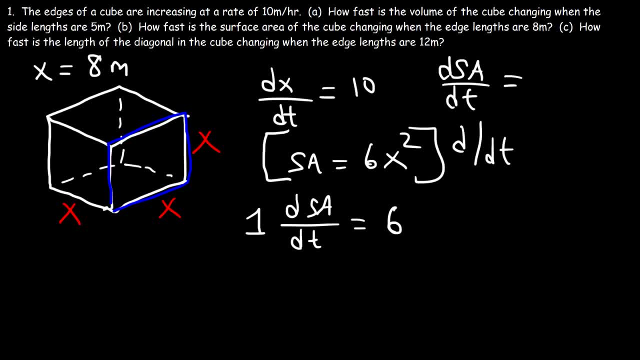 And then, for the right side, we need to rewrite the constant based on the constant multiple rule and then differentiate x squared based on the power rule, which is going to be 2x to the first power times dxdt. So 6 times 2 is 12, and then we can replace x with 8, well, let's put 8 meters. 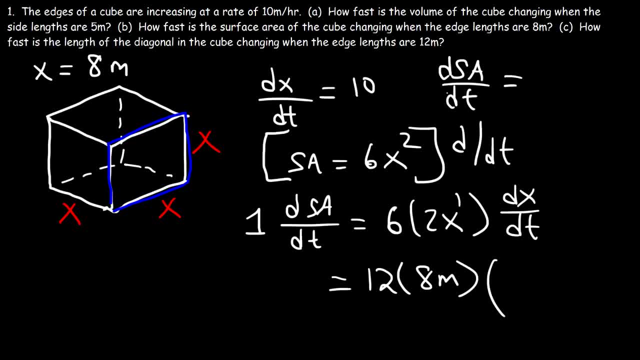 So we can pay attention to the units, and then dxdt, that's 10 meters per hour. So what's 12 times 8?? 10 times 8 is 80,, 2 times 8 is 16.. So 80 plus 16 is 95. 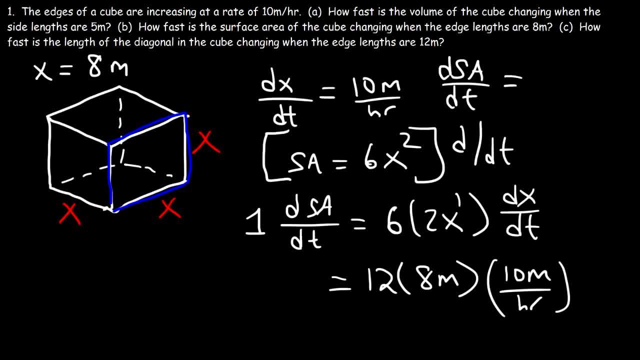 And so 12 times 8 is 96.. And then 96 times 10 is 960.. So dsadt is going to be 960.. Now, what are the units? So we have meters times meters, which is going to be square meters, and for dt it's going. 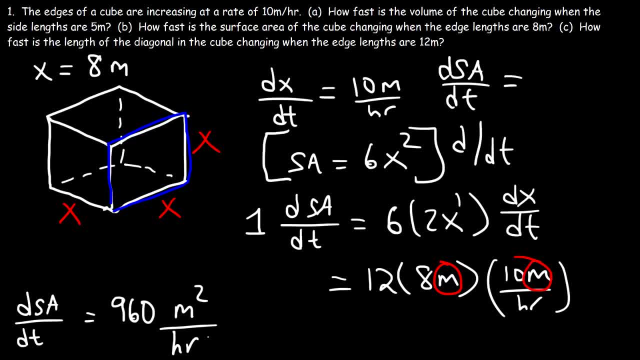 to be in hours, And it makes sense because the volume is usually in cubic meters. Area is going to be in square meters, which we do have here. So that's the value of dsadt: It's 960 square meters per hour. 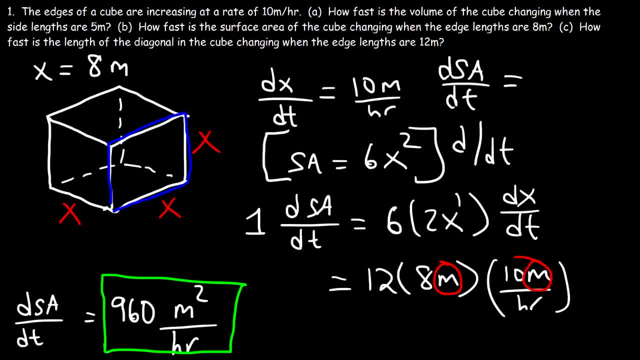 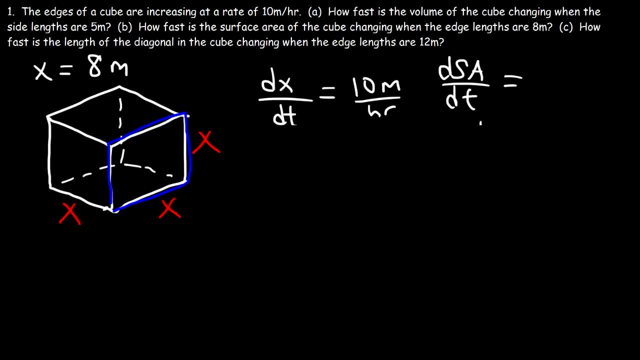 So that's it for part b. Now let's move on to part c. How fast is the length of the diagonal in the cube changing when the edge lengths are 12?? Let's replace this number with 12 meters. So first let's draw the diagonal that we're focused on. 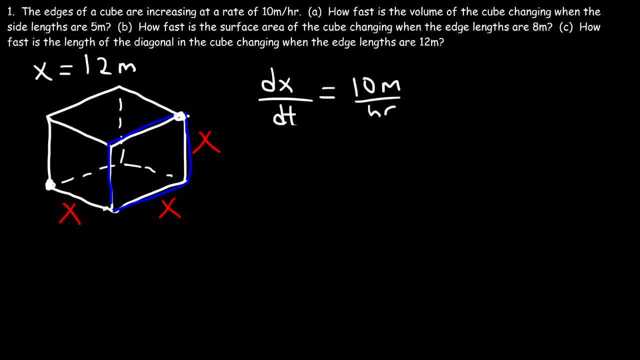 So it's the distance between these two points And I'm going to draw it in basically a red color. So let's call it z, diagonal z. So we're looking for how fast z is changing. So we need to calculate dzdt. 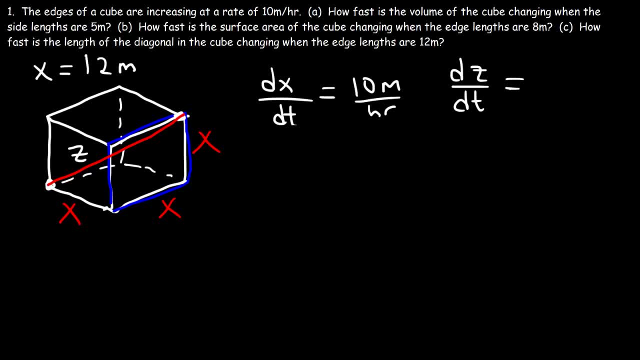 Now, how can we come up with an equation that relates the diagonal z to x? Now, first we need to draw another diagonal, which is going to be at the bottom face of the cube. Let's call that diagonal l. Notice that it forms a right triangle. 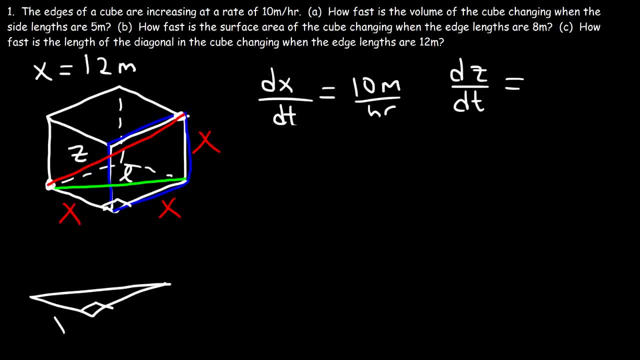 So, if you want to redraw it, it looks like this: So this is x, x, l. What is the relationship between x and l? Well, according to the Pythagorean theorem, which is c squared is equal to a squared plus b squared, c being the hypotenuse. l is the hypotenuse in this example, and a and b are. 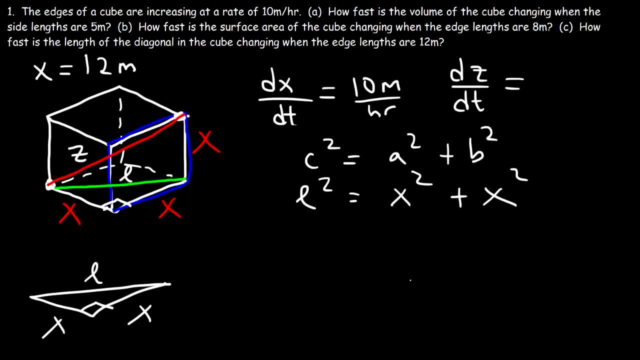 x. So l squared is basically x squared plus x squared. Now let's focus on another triangle which I'm going to highlight in blue, And that is this triangle. here Notice that it forms another right triangle, So I'm going to redraw it and for that triangle we have L at the bottom, X and Z. 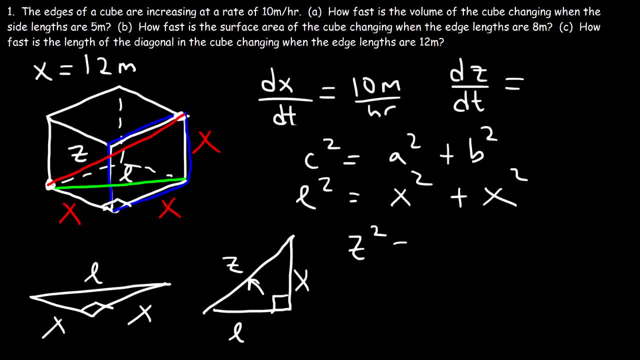 This time Z is hypotenuse. So this is: Z squared is equal to X squared plus L squared, And now we can replace L squared with X squared plus X squared. So therefore, Z squared is going to be X squared plus X squared plus X squared. 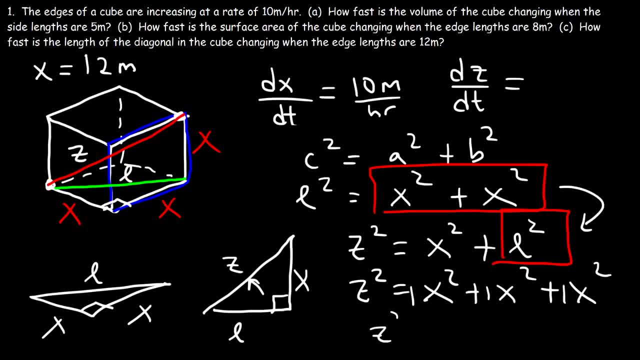 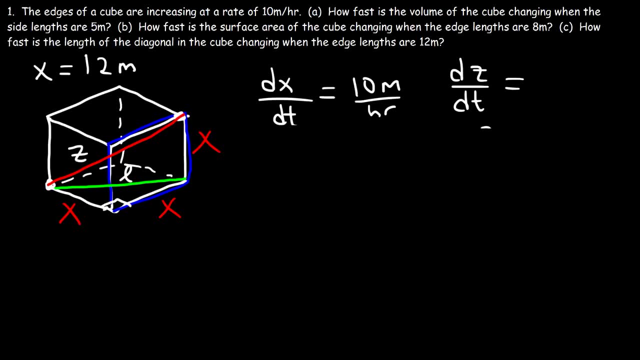 So 1 plus 1 plus 1 is 3.. So Z squared is equal to 3 times X squared, And so this is the equation that we need to relate Z and X. Now let's go ahead and find the derivative of both sides of the equation, with respect, 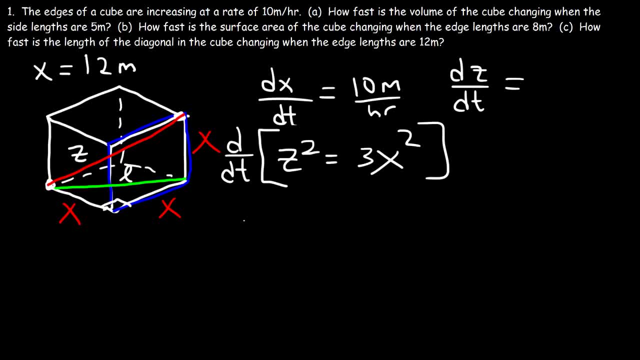 to T. So the derivative of Z squared is going to be 2Z times DZDT And the derivative of 3X squared is going to be 3 times 2X times DXET. So now we can calculate DZDT. 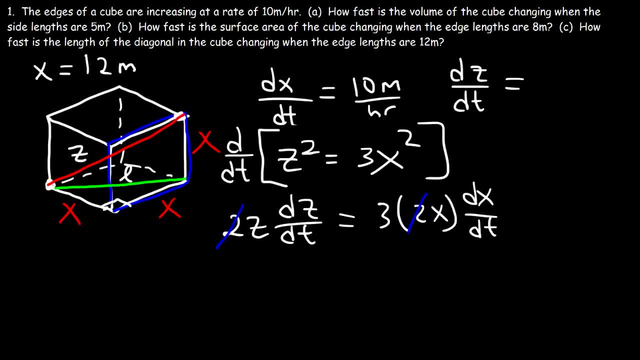 Okay, But first let's divide both sides by 2, just to get rid of that 2.. Now we need to find Z as well, because we don't have that. So let's use this equation to get Z. So we know that Z squared is equal to 3 times X squared. 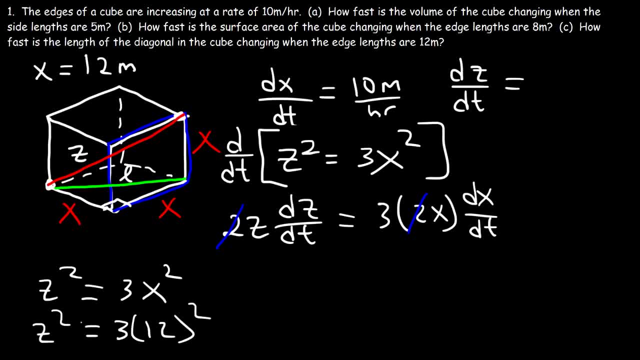 And in this example, X is 12.. So I recommend taking the square root of both sides at this point. So Z is going to be the square root of both sides. So Z is going to be the square root of 3 times the square root of 12 squared. 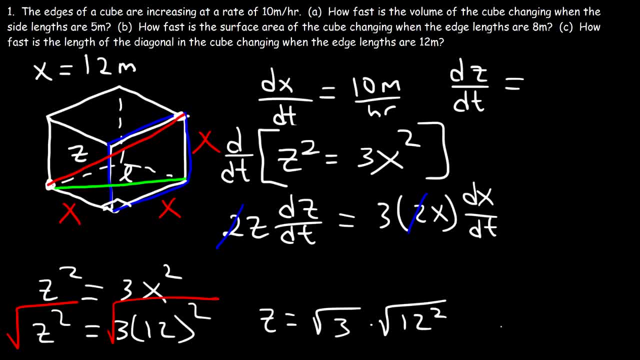 The square root of 12 squared is the square root of 144, which is 12.. So Z is basically 12 times the square root of 3, which I'm going to write over here Now let's plug in everything. So this is Z 12 square root 3.. 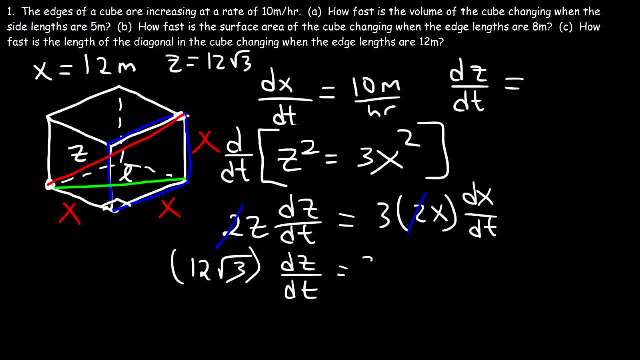 We need to solve for DZDT, And then we have 3 times X, where X is 12.. And then DXDT and that's still 10.. So if we divide both sides by 12, we can get rid of this.